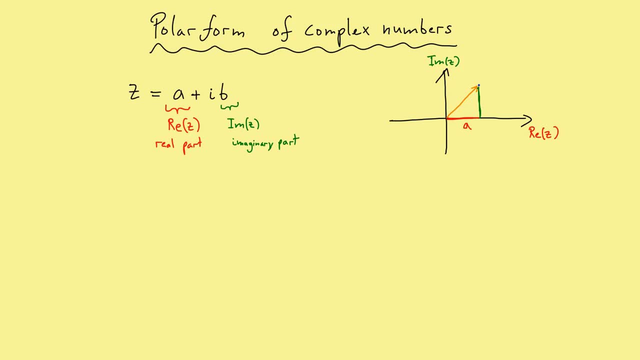 This means that this would be A and this would be B. So the real numbers A and B Build the complex number As a vector. So we could write it as a column vector, As usual in a two-dimensional space. So A and B in a column vector. 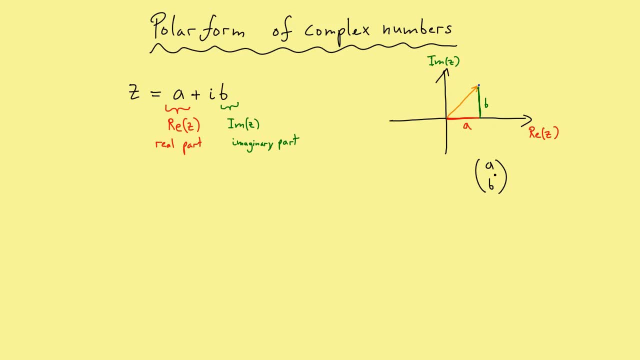 But for complex numbers we have a better term to write these things. We use this notation. So the first entry is just A, So it gets nothing else, But the second entry gets the I in front. This is very useful for calculations. We can just multiply and add the things like normal numbers. 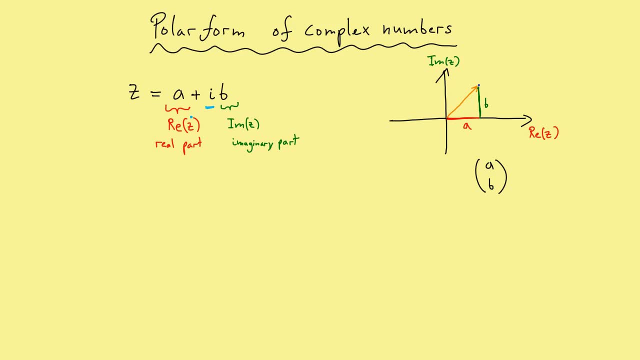 So we can do all calculations we know, for the real numbers, for the complex numbers as well, And we just have to use that: I squared is minus I. Of course this is an important equation And it just means you would do all calculation as usual. 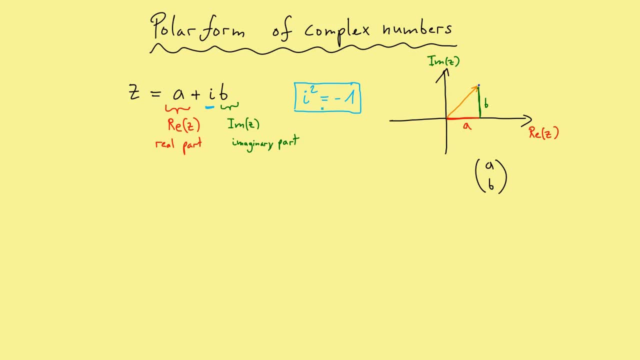 And every time you have a power of I, You use this formula And in the end you get again a complex number with a real part, And I times an imaginary part. So now I want to use this picture. Maybe I will do it in a larger form. 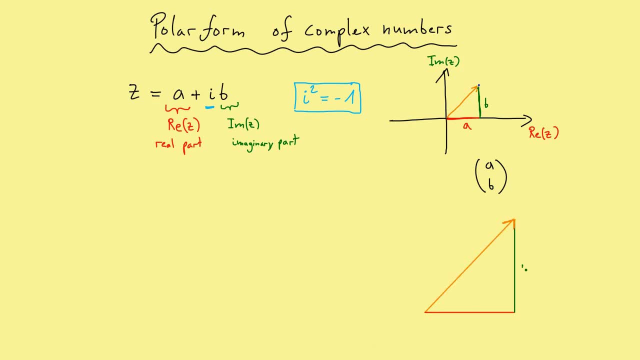 There we go. So we have here B, And the real part is A. here, Of course, our vector, our complex number Z, Is uniquely given by the two components here And of course we have a right angle here. So, as you can see, 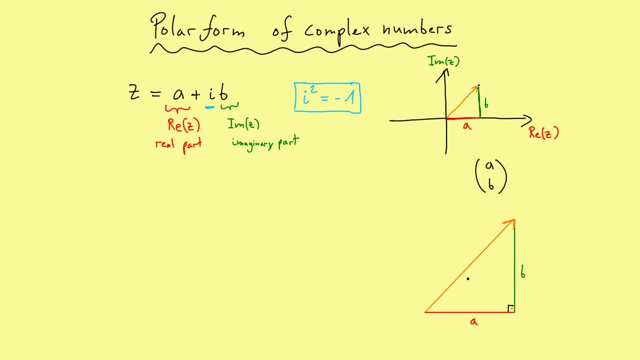 Of course we could just determine this vector or the complex number If we know two other things, For example, if we know this angle here From the x-axis to the y-axis. So in positive sense I would say, So we know the angle to the x-axis. 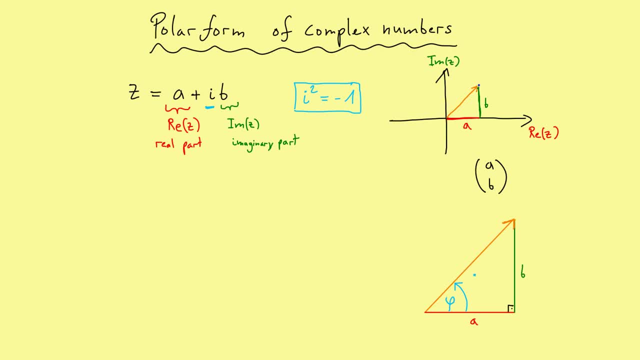 And I call it just phi. And if we know the length of this vector, So the length, we give the name r. So if we know these two values, We also get this point here. So by knowing how much we have to go in this angle, 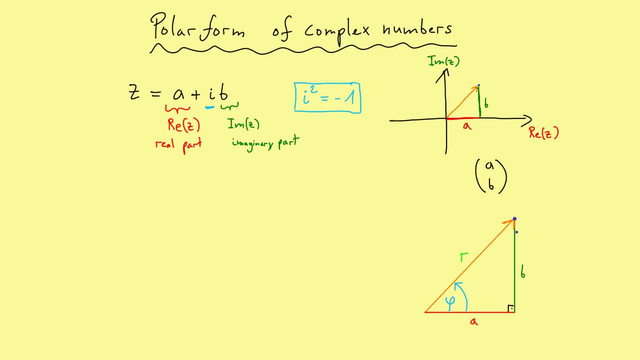 And the length of this vector. We get this point Uniquely And in the right angle triangle We can use Pythagoras And this means That this side is given by r and the cosine of phi And the other side here. 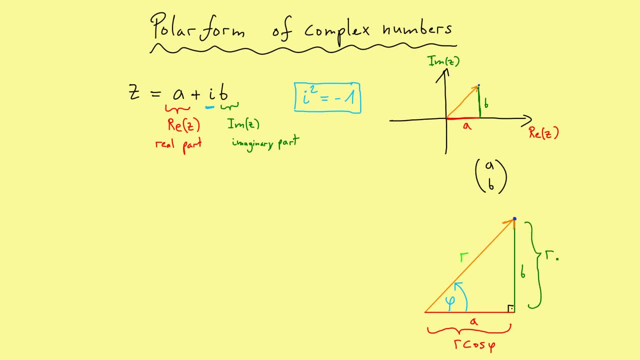 Is given by the sine of phi, So r times, sine of phi. And then we get immediately the polar form of the complex number And we can say: Okay, we put this r times cosine, So r times. And here we get the brackets. 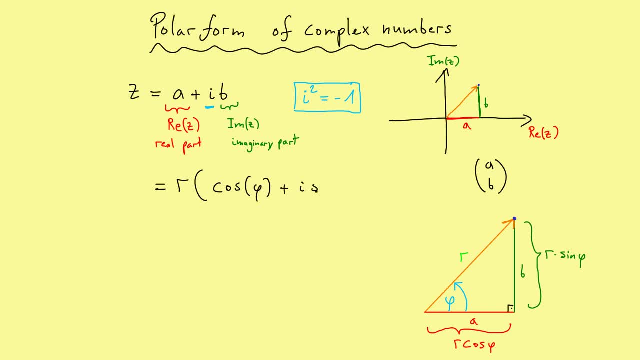 Cosine plus i sine of phi. Well, this is very easy to see And, as you can see, We have now two other values we can put in: An angle phi And a radius r. So now it's not so easy to see. 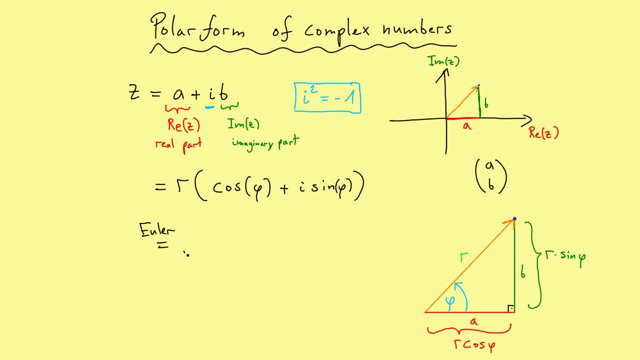 That we have the Euler identity. That means This is just given as an exponential function. So instead of writing Cosine phi plus i sine phi, We can just write E to the power of i phi. And this thing is what we also call. 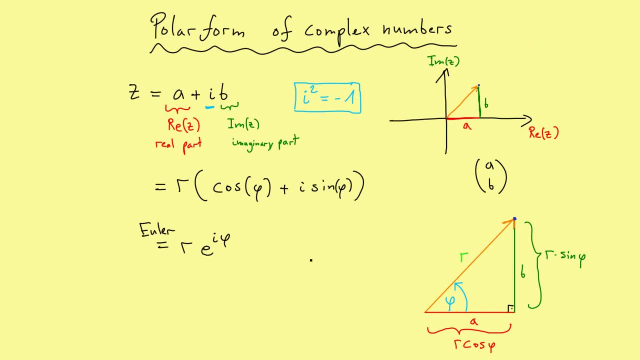 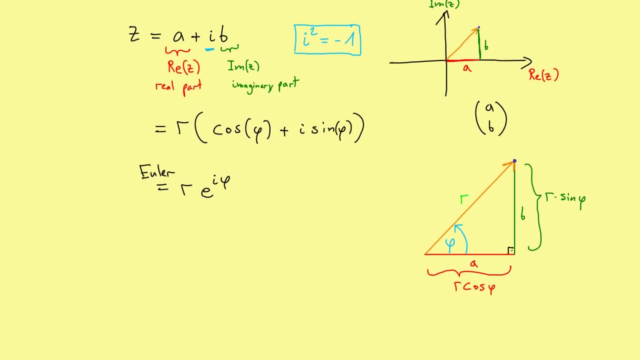 The polar form of a complex number, Since it's the same meaning. We need an angle And a radius, r. A good question is now: How do we get these numbers If we have the real part And the imaginary part? So we need a formula. 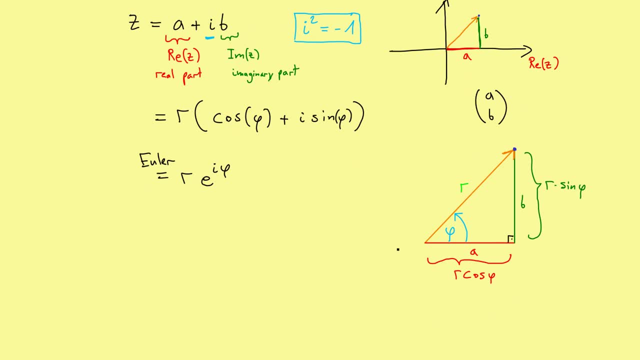 For calculating r And phi. Okay, before I said We need Pythagoras here. Okay, it was just a definition of cosine and sine, So it was not really Pythagoras, But of course it's a right angle triangle So we can use Pythagoras. 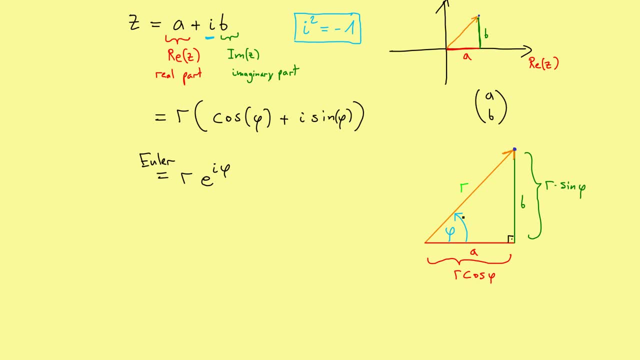 And this means Our r. The length of this side here Is given by the squares And then the square root of this side. So just writing: r Is equal to the square root Of a squared Plus b squared. This is in real Pythagoras now. 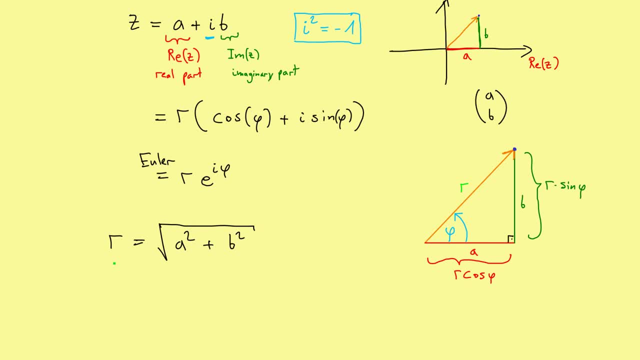 Well, getting r, So the radius, Is not very hard, as you can see. You can just square These real numbers And take in the root. That's not so hard. But getting the angle, Yeah, there we need Some roots. we have for sine and cosine. 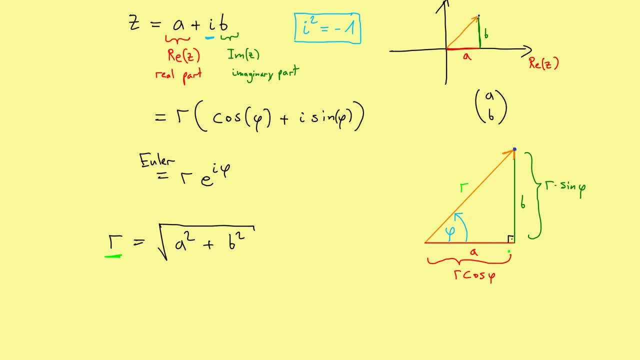 So of course, we can use just that: The cosine is this side Divided by this side, Or the sine This side divided by this side. However, of course, We just want to use The x of the right angle Triangle here. 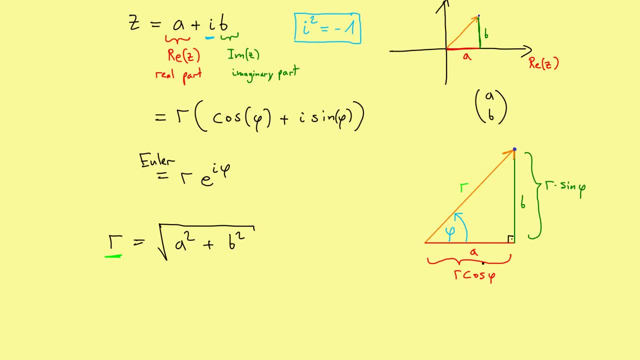 That's because They are given. So we have a and b given By the complex number. So we just want to use a and b And not r itself. We can use r after we have calculated, But maybe we don't have it. 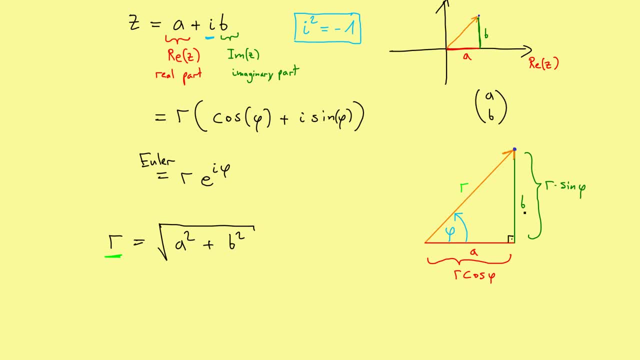 At the beginning. So we want the formula Just for b and a, And this means We need the tangent. So just tan of phi Is given By b divided by a, So b over a, So we immediately get The tangent of phi. 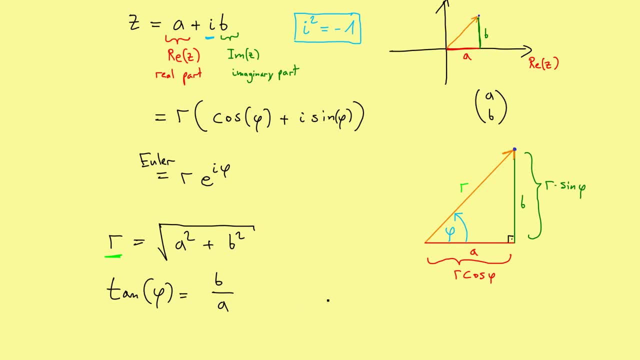 Just by b and a here. This should mean that we can Get the phi by the arc tangent, So arc tangent of b Divided by a. However, This is not quite true. We lie here In the interval Minus pi over two. 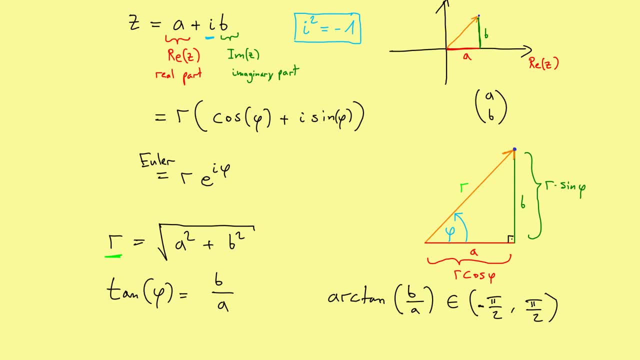 To pi over two. So the arc tangent Just gives us Angles between minus pi half. So this would be all Complex numbers In this half plane here But nothing else here. So this is not quite true, But of course. 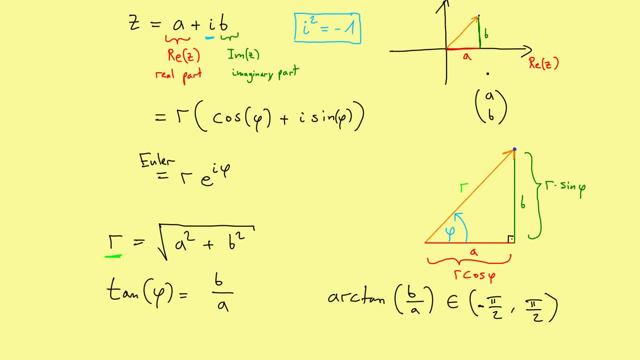 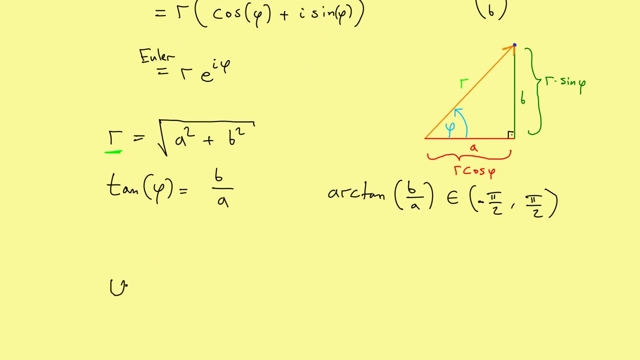 It should be true For the right hand side here And for the left hand side, But I explain it In more detail now. This means that we have to look At the plus or minus sign Of the wheel part, And then we can redefine. 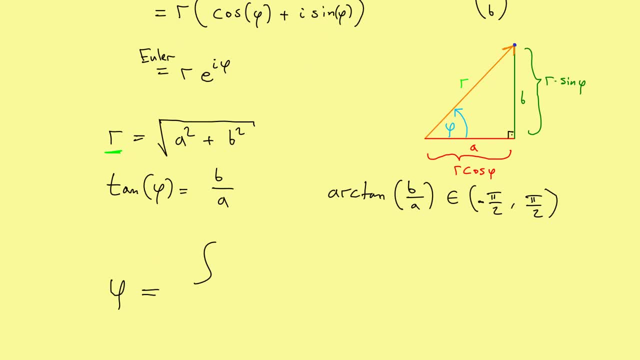 Our phi By setting. And now we look At the sign of The wheel part, So we define it as The arc tangent of b over a If The wheel part Is greater than zero. This means that We have all complex numbers. 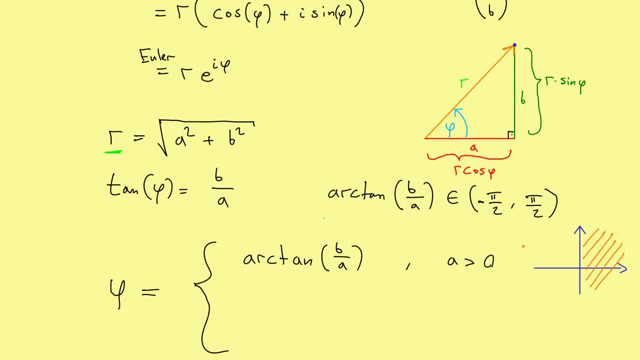 Here on the right hand side. So we get All angles between Minus pi half and pi half. So there is everything fine. So what happens If we have a vector Or complex numbers On the imaginary axis, So on the y axis? 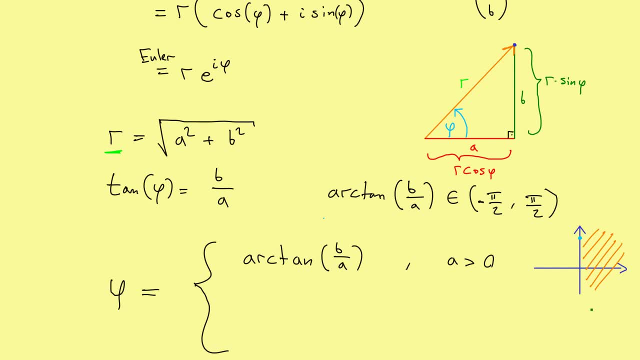 For example here The other part, Just here. So plus and minus Imaginary part. So then of course The wheel part would be zero. This formula is incorrect. Of course we divide by zero. That's not good, But of course we know the angle. 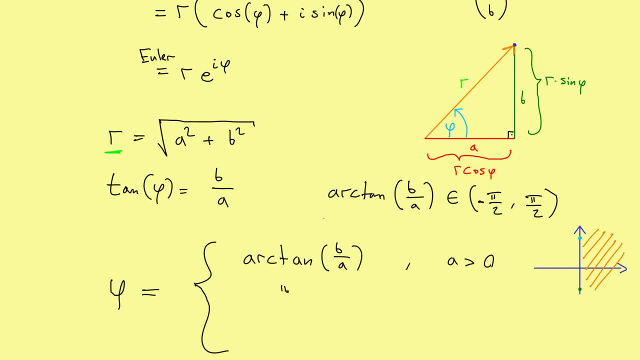 For this number here, For each number on the positive y axis, It's just pi over two, Just the right angle, So pi divided by two. So this is very easy. We can just define it And see immediately. We don't have to calculate. 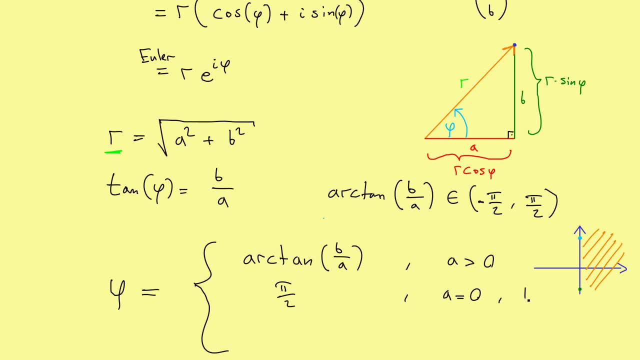 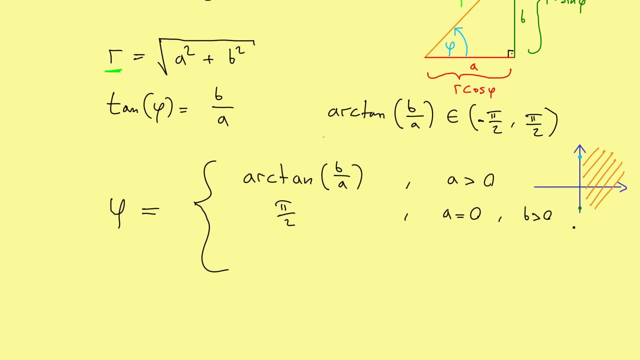 The angle is clear. So for alpha equals zero And positive b, We have this angle, And for the negative B, So it would be the same. Okay, we could say: This is just Three times pi divided by two, So just. 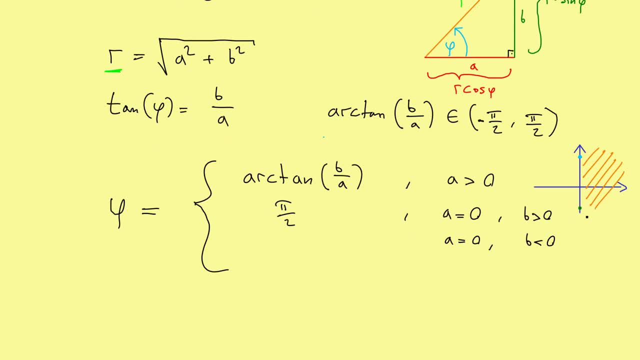 Three right angles. But of course we can just Use the negative value here, As we used here before. So this would be minus pi over two. So we can do the colors here. So we get the whole axis here With the blue part. 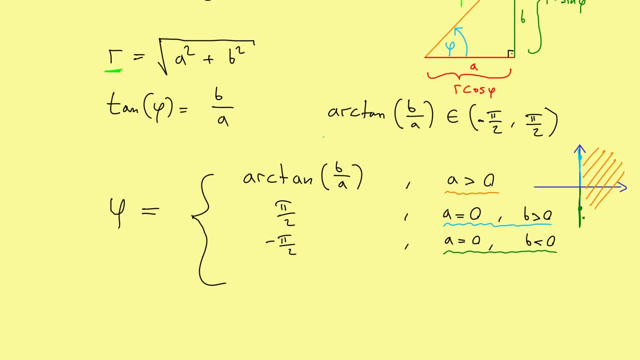 And the green part With the y axis here. Okay, So just missing Is the left hand side here, And this means We have a negative. The real part is negative, The imaginary part could be positive or negative. So now, 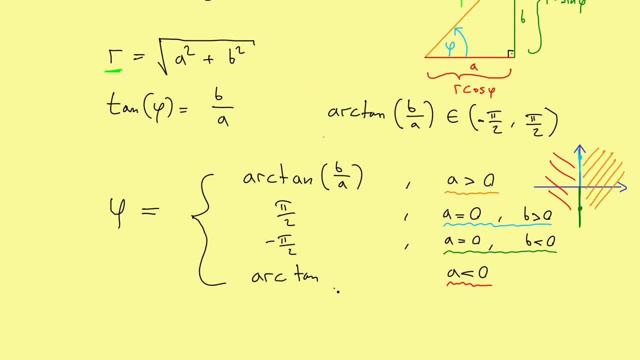 If we use the same formula, So arc tangent Of b divided by a. This is well defined, But we get a value In this interval. So for example, If we choose a vector here, So for example This one here: 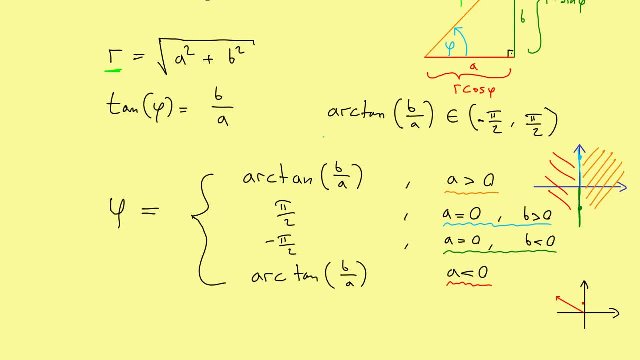 You see, okay, We have a negative real part But a positive imaginary part, But then we divide These two numbers, So we have a minus sign here, But it is the same As we have the minus sign If we have the minus sign. 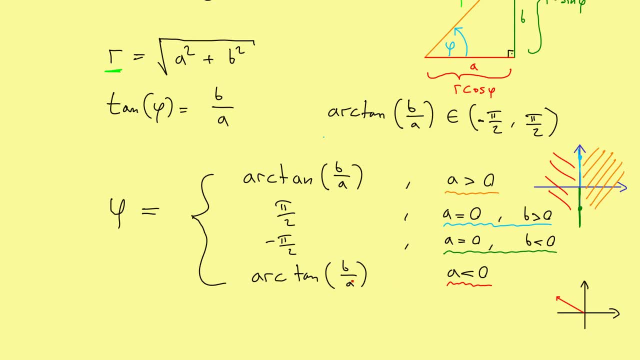 On b. The value here is the same. Minus sign is just In the denominator Or in the denominator. Therefore We don't get the angle here That we want. So, as we can see, This would be the same as calculated. 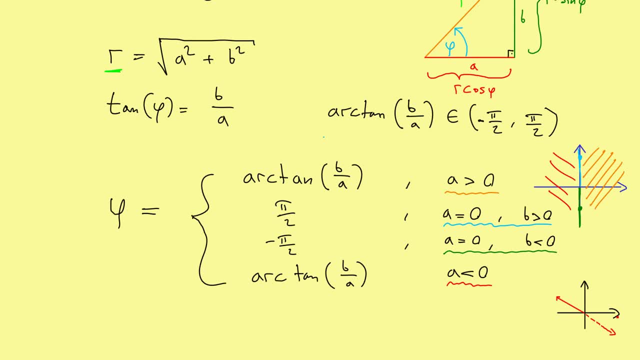 With this vector here. So then we have just switched the signs From b to a, But this is For this formula here. So we get this negative Angle here By using this formula And, as you can see, We have just switched sign. 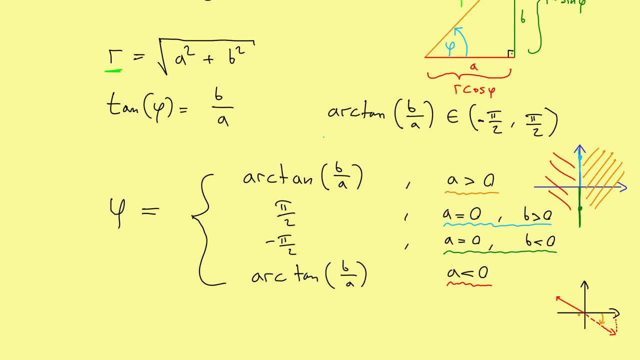 So the real angle is off By exactly one half circle, So by exactly pi. So by adding Just this pi We can get The wanted Angle here. So we have this angle. Putting pi At pi, We have the wanted angle. 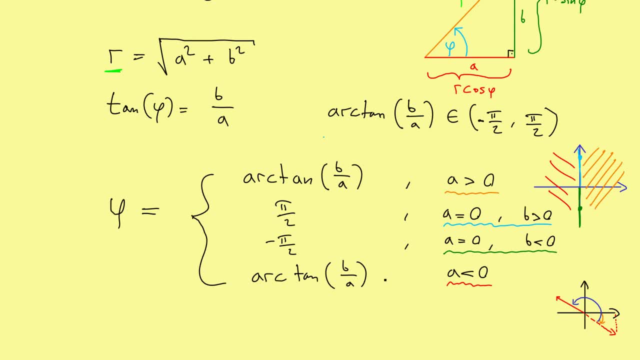 We get this vector. So just put in plus pi And that is correct. And the same works On the negative imaginary part as well. Then we can just mirror These two vectors. As you can see, Calculating the polar form of complex number.